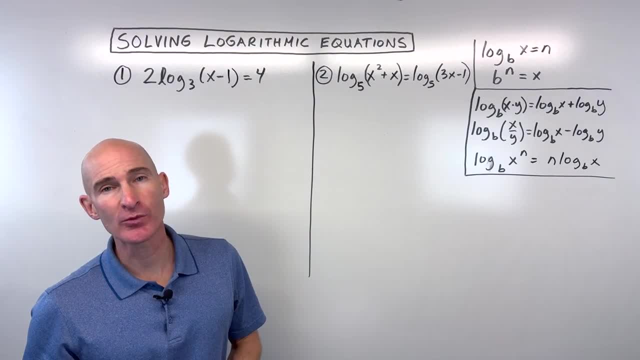 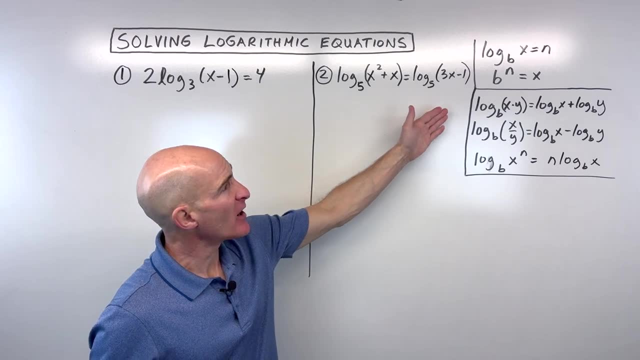 In this video you're going to learn how to solve logarithmic equations and we're going to go through five examples together. I'm going to give you some pointers along the way. Let's dive into this video. The first thing we want to talk about, or just review, is some key concepts with logarithms One. 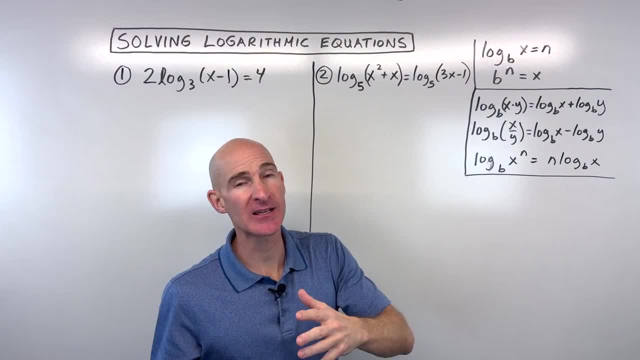 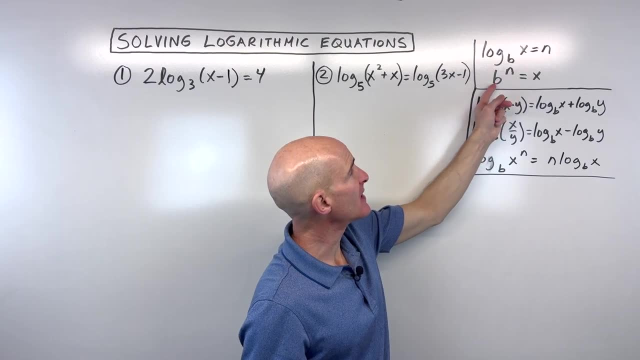 is how to switch back and forth between the logarithmic form and the exponential form, and that's what we can see here. We've got log: base b of x is equal to n. We can write that as an exponential function by saying: the base b raised to the nth power is equal to x. So you can switch. 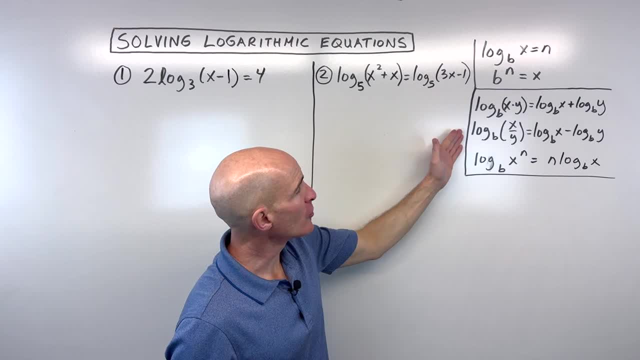 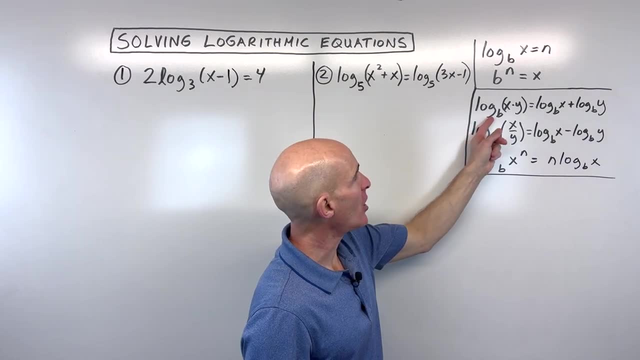 back and forth between these two forms. and then you want to learn the expanding and the condensing properties, So how to expand logs and how to condense logs, and so that's what this illustrates here. Log base b of x times y. We can write it as the sum of two logs, Okay. log base b of x plus log. 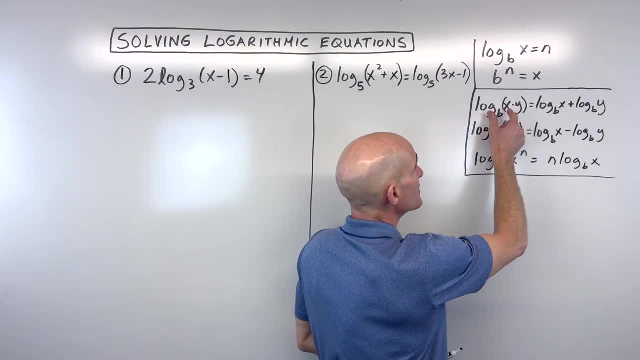 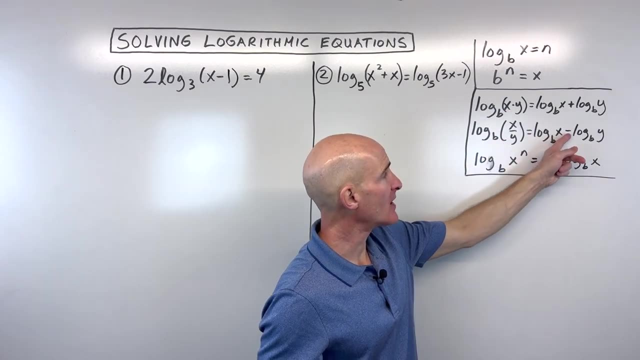 base b of y, or we can go from the right side to the left side, where we're condensing it into one logarithm by multiplying that When we divide we write it as a difference of two logs. and when we have this power, we can bring: 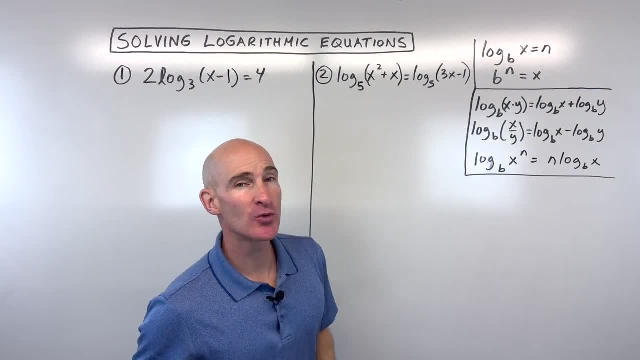 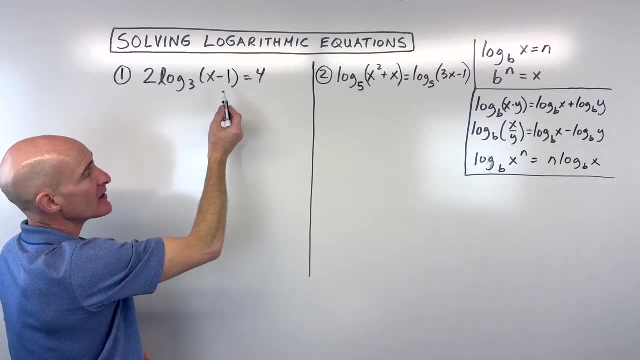 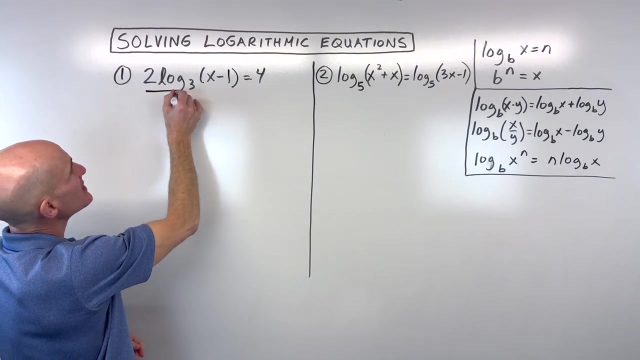 this power down in front of the log. So I'll show you how these work as we get into these examples. but for the first example, we've got two log base. three of x minus one is equal to four. How do we solve for x? Well, what we can do is we can start off by dividing both sides by two. 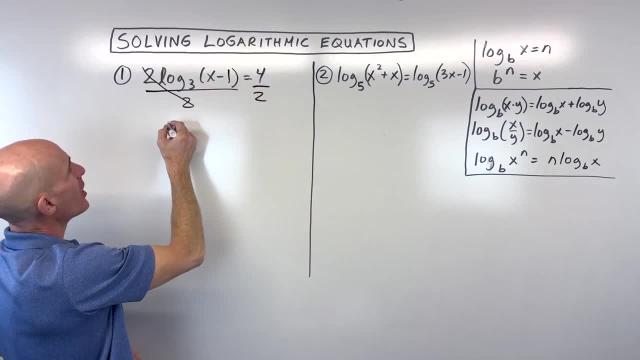 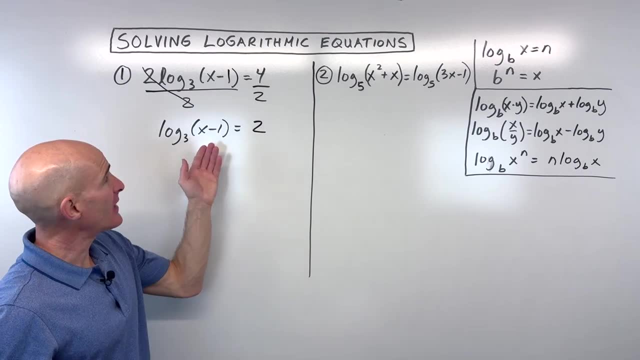 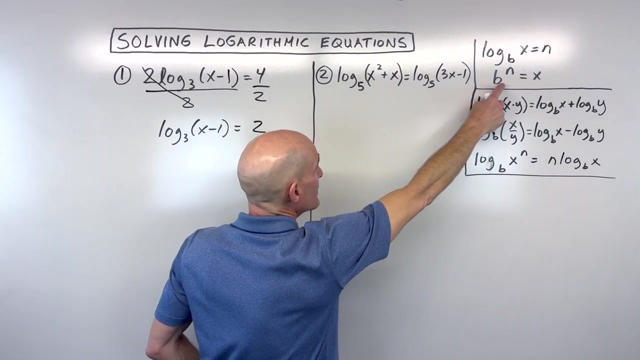 to get this logarithm by itself. So we've got log base three of x minus one is equal to two. Now you see how that variable is kind of like inside of that log. We want to get it by itself, and the way that we can do that is by rewriting it in the exponential. 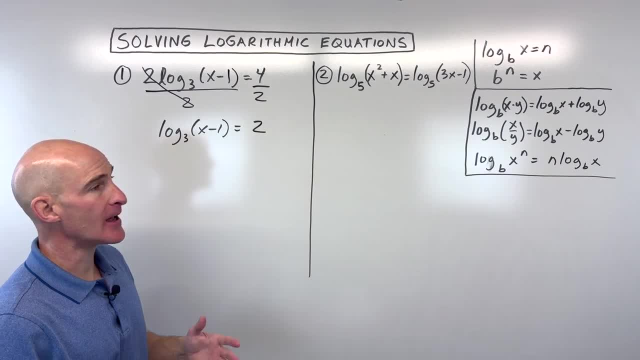 form. Now, an easy way to think about this is that exponential functions and logarithmic functions. they're inverses of each other. So what we can do, if this is log base three, we can quote, unquote, exponentiate both sides or raise both sides using base three. This is a very easy way to do it. 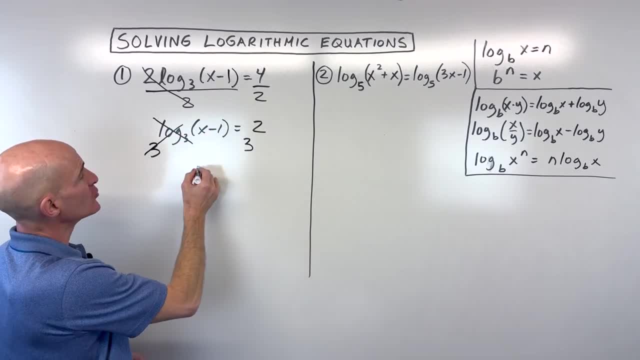 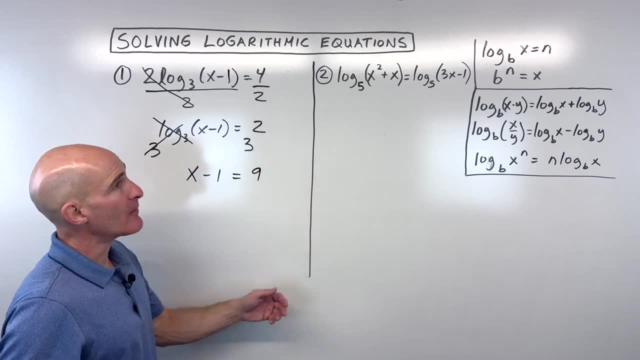 This is a nice way to kind of think about them, as being inverses and undoing one another, leaving us with this argument here: x minus one is equal to three squared, which is nine. Now, if you don't like that method and you just want to utilize these formulas here to switch the forms, that's completely. 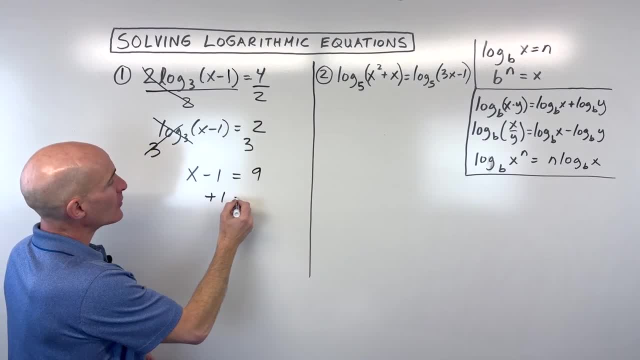 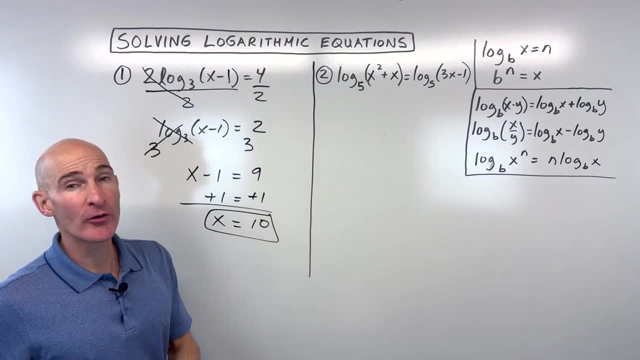 fine, This is just another way to look at it. and then, lastly, we're going to add one to both sides and you can see we get x is equal to 10.. Now, when you're working with logarithmic equations, it's good to take your answer and put it back in. You can see that you can get x is equal to 10.. 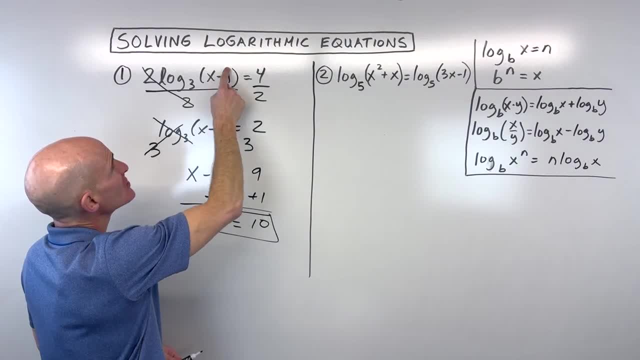 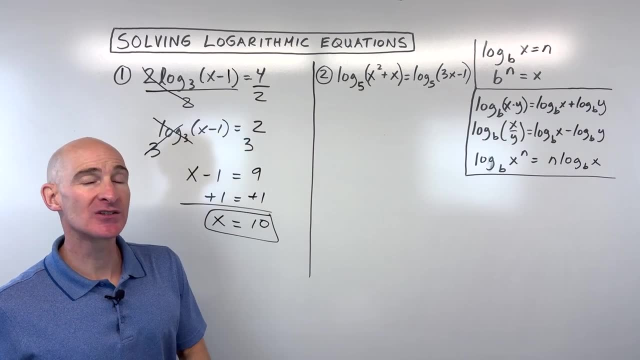 You don't have to solve the whole equation, but you want to make sure that this quantity here is positive. It shouldn't be zero or negative. If it does come out to zero or negative, then it's an extraneous solution and you would then cross that out. There would be no solution, but in this case, 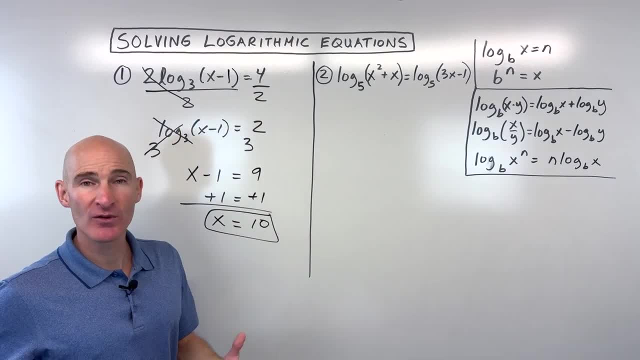 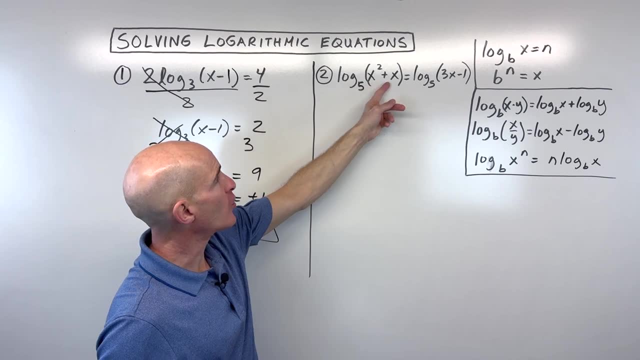 you can see, 10 minus one is nine. That's greater than zero. We've got a good answer there. Okay, let's go on to example number two. now, Here we've got log base five of the quantity x squared plus x is equal to log base five of three x minus one. How do we solve that? 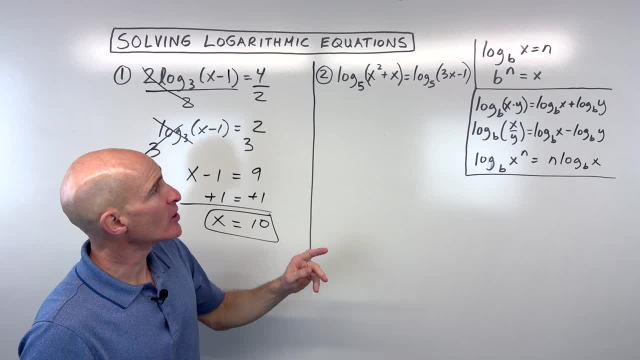 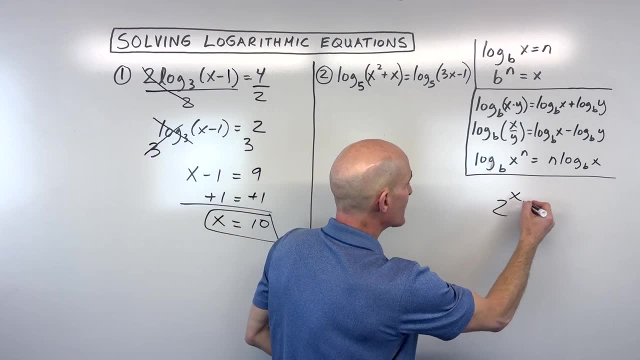 Problem, So a little bit different than this first one. This is what we call the one-to-one property of logs. You probably learned the one-to-one property of exponents, like if I had two to the x, is equal to two to the y. then see, they have the same base, so we can set the powers equal Well. 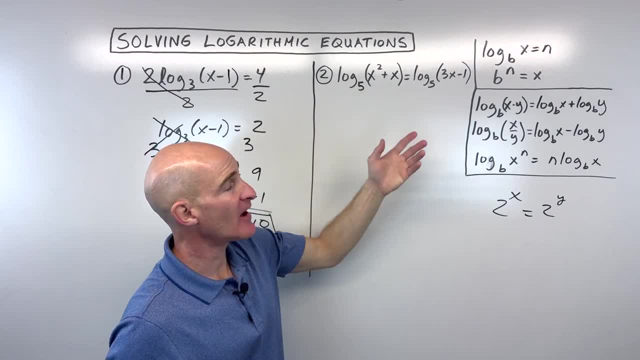 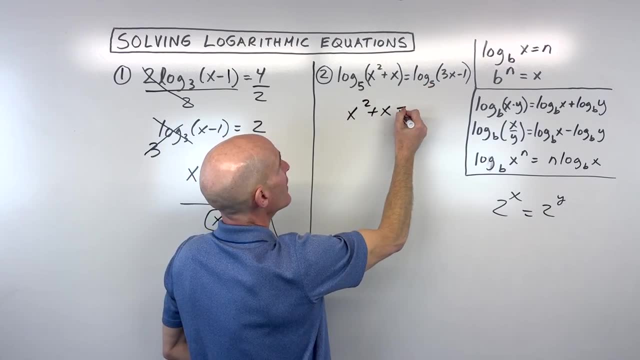 it's the same thing with logarithms: If you have log base five, log base five, those two logs are equal to each other. that means that these arguments here must be equal to one another. So we're going to set those equal to each other here. 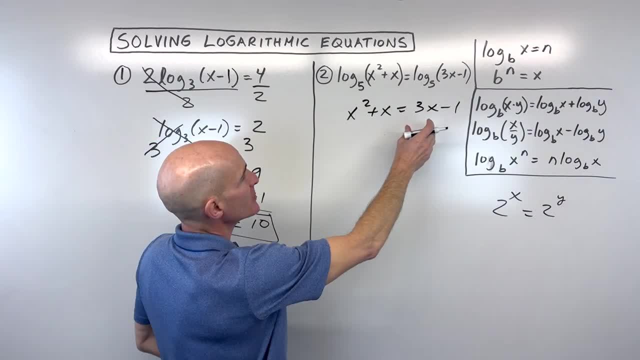 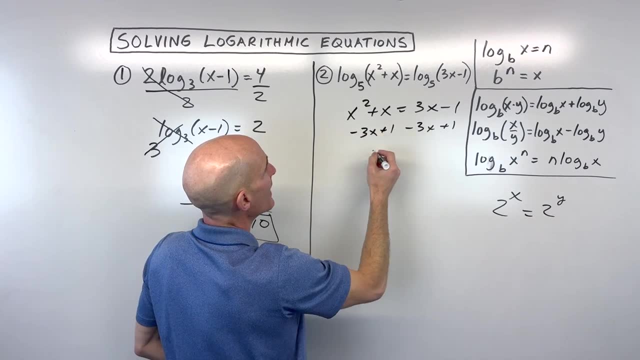 And now you can see we have a quadratic equation, a second degree equation. Let's go ahead and get everything on one side of the equation and set it equal to zero. So I'm just going to add one to both sides and subtract three x from both sides, So that'll give us zero on the right and on the 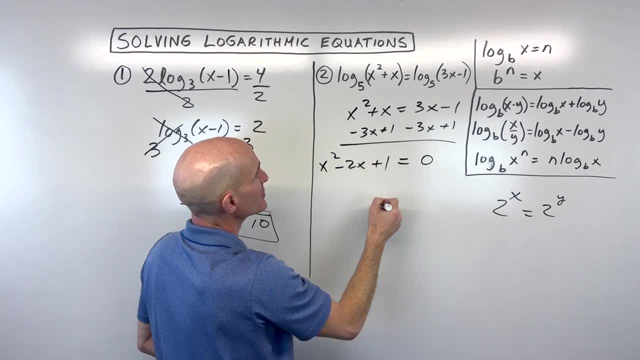 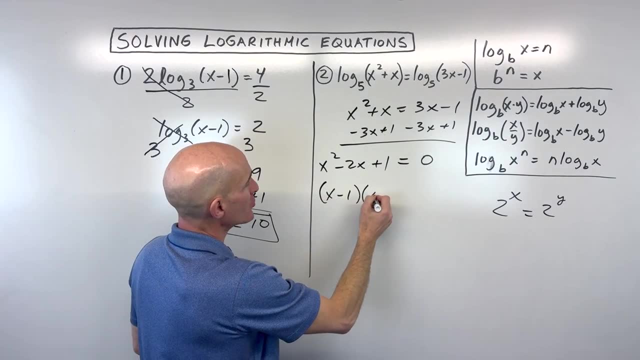 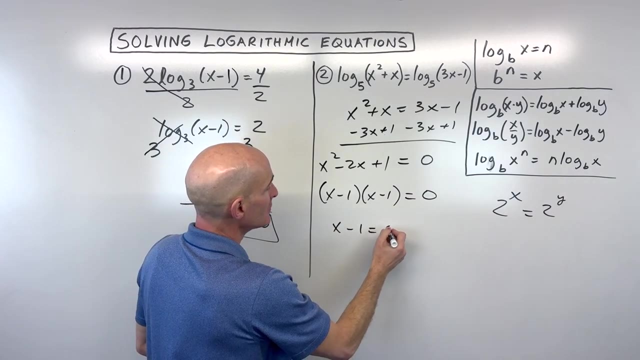 left, we have x squared minus two, x plus one. Okay, so now what we can do is we can factor this and this factors to x minus one squared, or you could say x minus one times x minus one, And by setting both of these factors equal to zero, you can see that we're just getting x equals one. 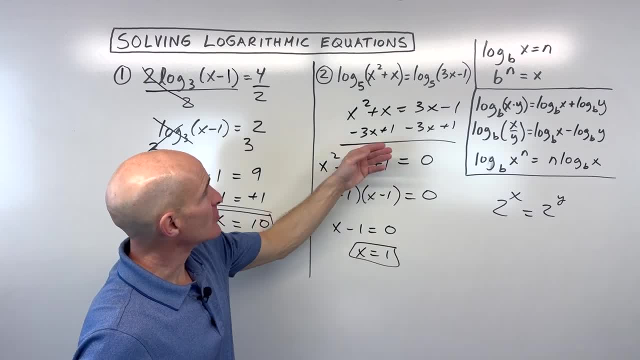 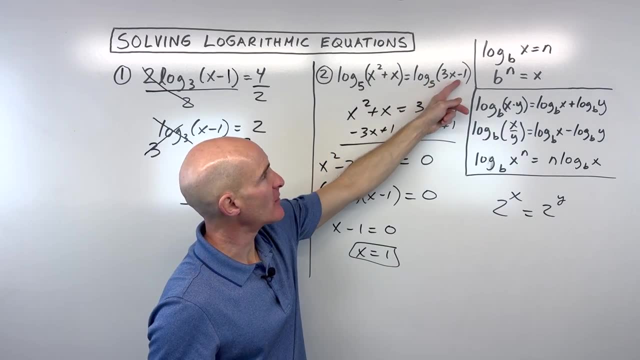 twice Okay. well, again, we want to take this answer and put it back in, make sure this comes out to a positive value. We have: one squared is one plus one is two. Three times one is three minus one is two. You can see: log base five of two is equal to log base five of two. Again, we want to make sure. 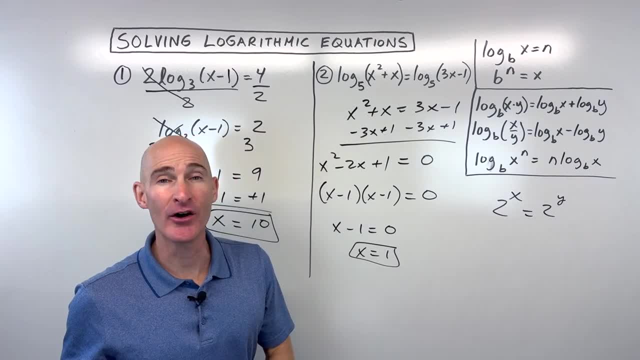 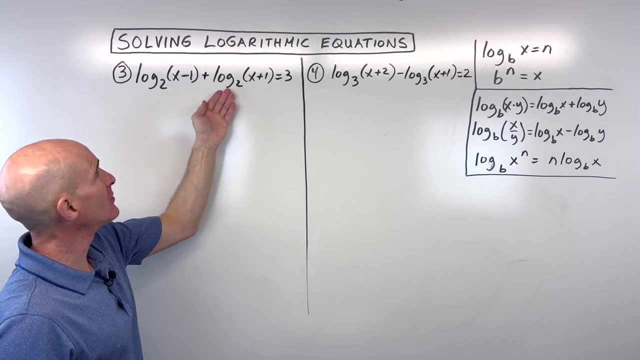 that this quantity doesn't come to be a zero or a negative value. Let's take a look at some more examples. Okay, let's go on to example number three. now We've got log base two of x minus one plus log base. two of x plus one is equal to three. So how? 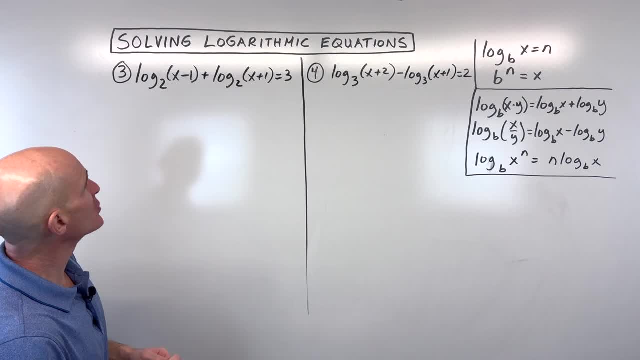 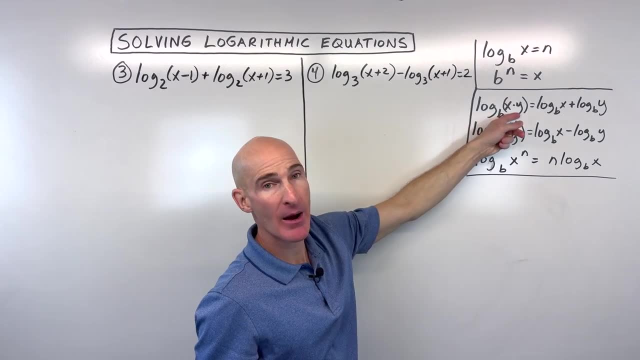 do we solve for x in this equation? Well, what we're going to do here, we're going to utilize another technique, and that's to condense these into one log. So we're going to be using this product property of logs, where, when you have a sum of two logs, as long as the bases are the same, 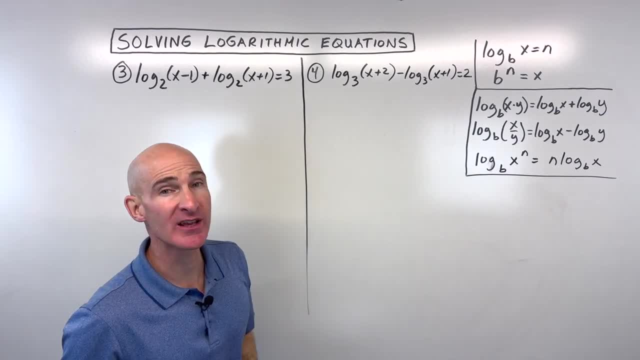 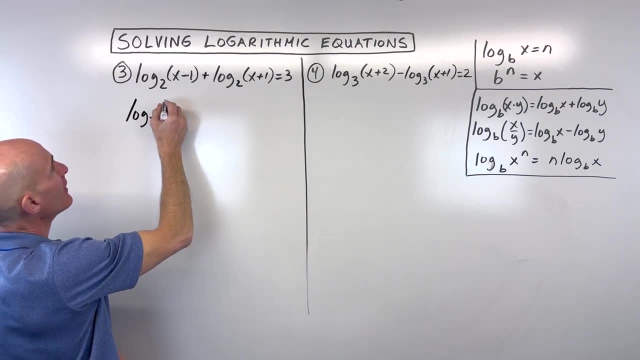 we can combine them into one log by multiplying those arguments x and y together. So in this case, that's what we're going to do. We're going to condense this into log base two of x minus one times x plus one. Okay, so I'll just do this in two steps here. So x minus one. 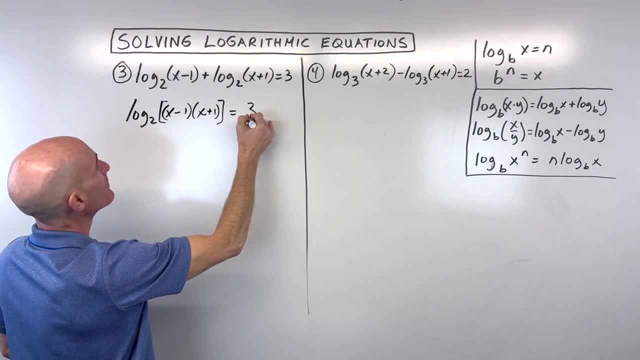 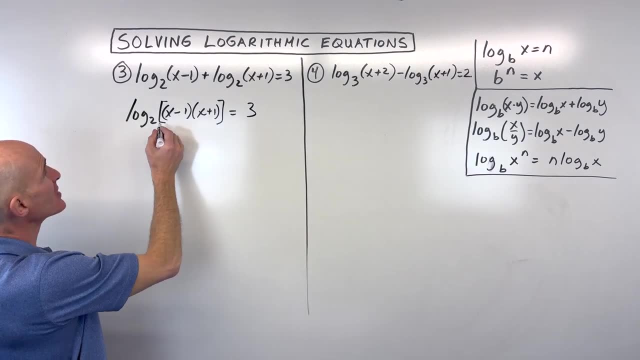 times x plus one is equal to three. Now, when we multiply these together, you probably recognize this as a sum and difference pattern, which is going to come out to a difference of two squares. If not, you can FOIL it out or distribute twice. We're going to get here log base two of the 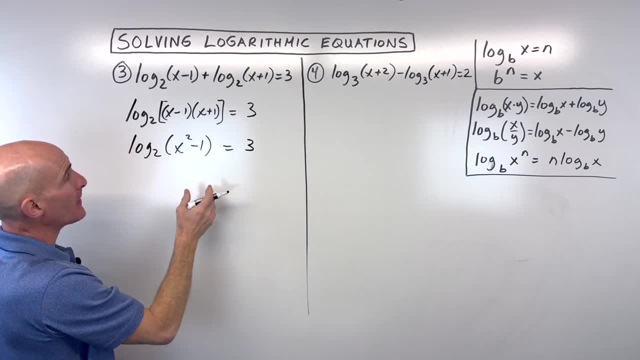 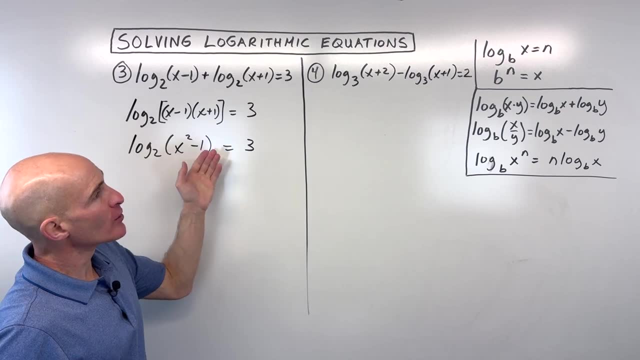 quantity x, squared minus one, is equal to three. Okay, so now that we've condensed it, we can see our variables inside of this logarithm. So we want to get this by itself. What we're going to do is we're going to use this technique of rewriting it in the exponential form, The way I like to do. 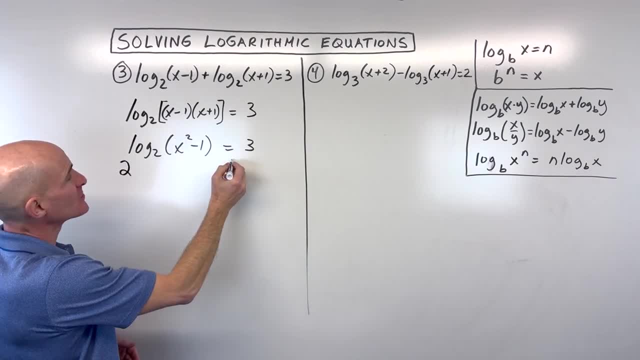 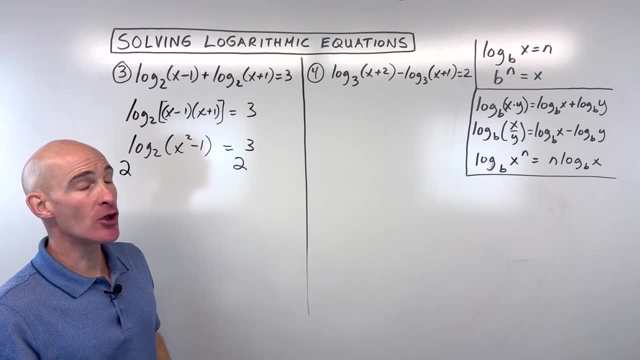 it, just because I like to keep things simple, is I like to think about exponentiating both sides, because the log rhythmic function and the exponential function, they're inverses of one another as long as these bases here are the same. So what happens? these undo or cancel each other. 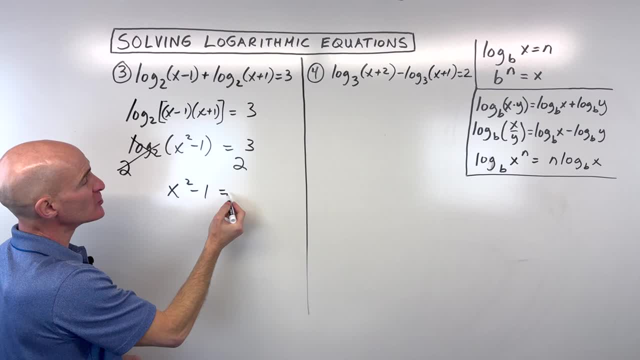 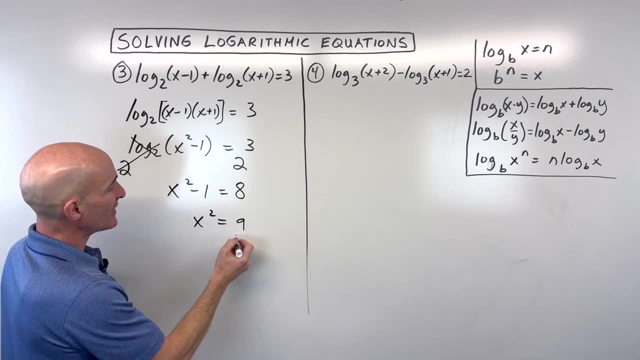 out and we're left with here: x squared minus one is equal to two, to the third power. Two times two times two is eight. Let's add one to both sides. That's going to give us x squared is equal to nine. It will take the square root of both sides. Remember, when you take the square root of 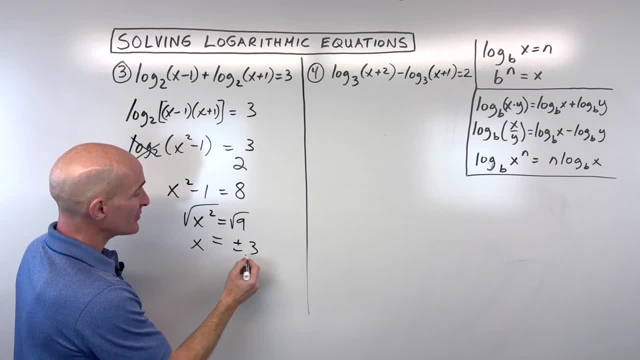 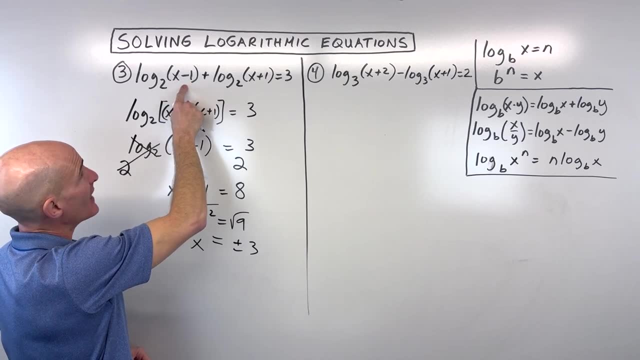 both sides. you get two answers plus or minus, and the square root of nine is three. Now what you want to do? we always want to go back and check. So if I put negative three in for x, you see how we get negative four. We can't take the log of a zero or a negative number, So negative three would be. 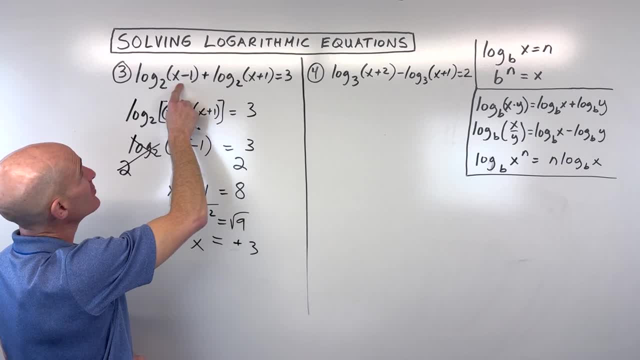 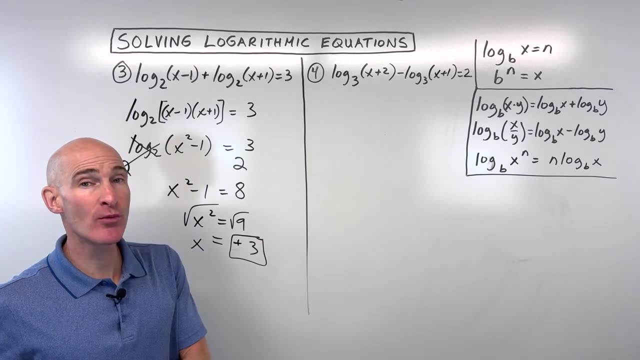 extraneous. and let's check positive three. Three minus one is equal to three, So we're going to take negative. three plus one is two, That's positive. Three plus one is four, That's positive. So in this case we're just getting the one solution of three. So super important, you can see. 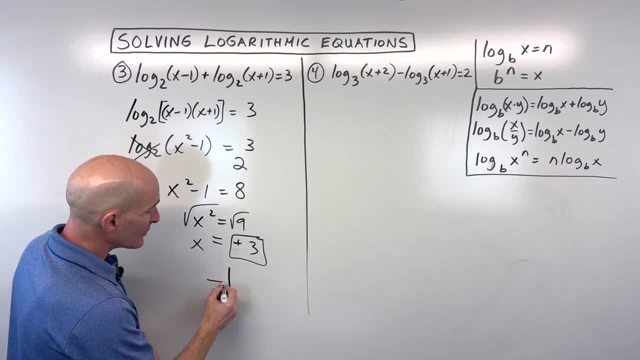 to go back and check. If you want to look at the graph of logarithms, just a basic graph of a log function, it looks like this: It's going to be approaching that y-axis, Okay, but notice how it doesn't cross the y-axis, It doesn't touch the y-axis and it's not to the, to the left here. So 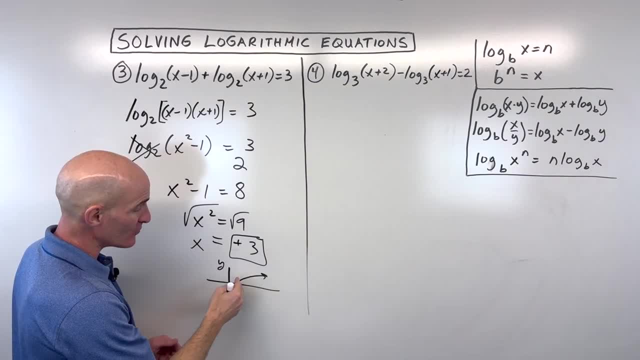 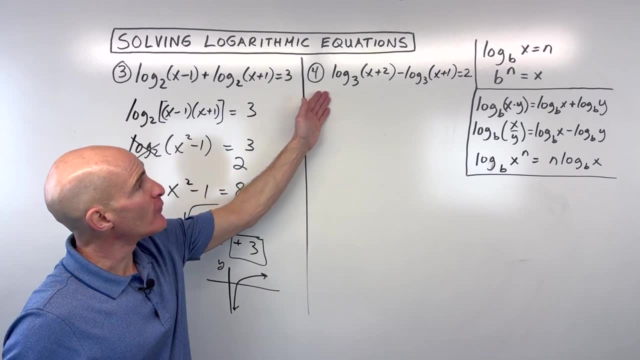 you can see, these inputs or these domains, or the x values are going to be greater than zero. That's why this argument here: we want to be a positive number. Now, before we dive into number four, if you enjoy the way that I explain things and you want to learn more about algebra one, 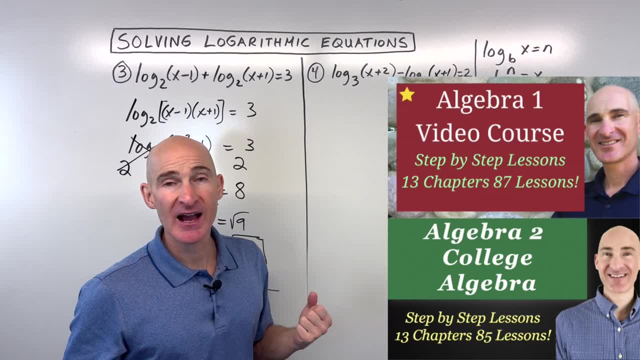 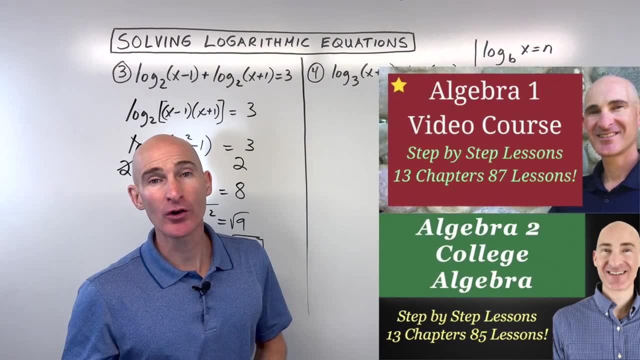 algebra two, college algebra, where I talk about a lot of these concepts with logarithms as well as many other topics. check out my links in the description below to my courses where I go step by step, building on one concept after the other, and check out those. courses are for sale. 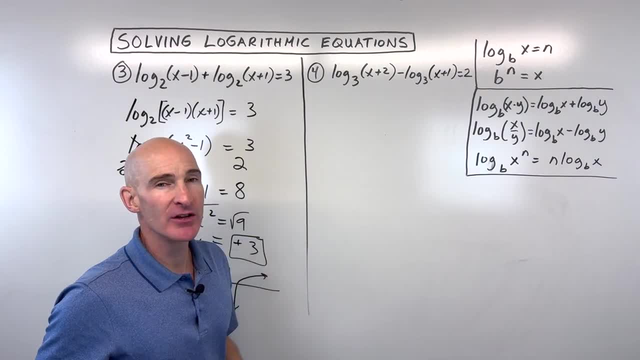 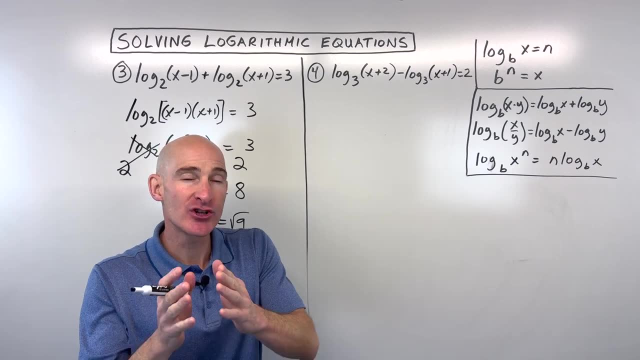 Number four. now we've got two more examples and I'm trying to show you when I go through these videos. I don't know if you notice this, but I try to start kind of easy and I try to build on those two more challenging concepts and I also try to show you the different types of problems that 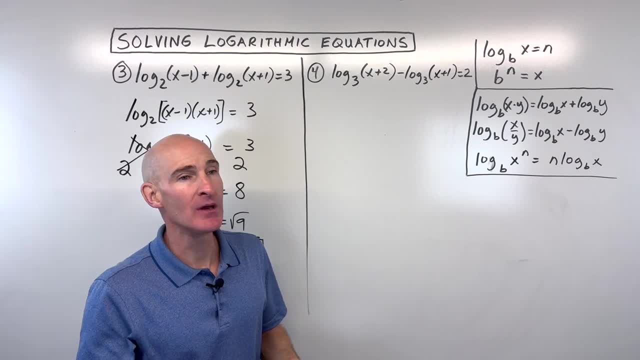 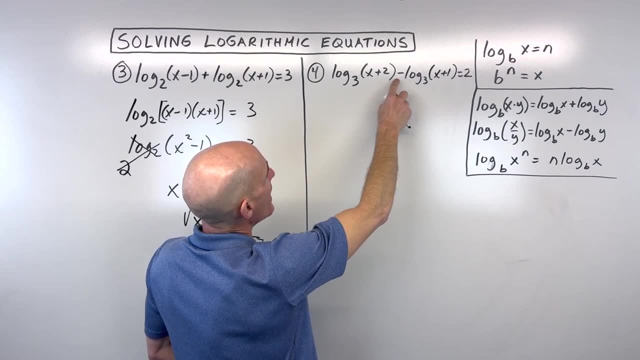 you're likely to encounter. I usually don't give you a lot of the same problem, but I want to give you a variety, so you really know how to to tackle these. So for number four, notice, here we're subtracting these two logs, right. So what we can do is very similar to this last example, but we're 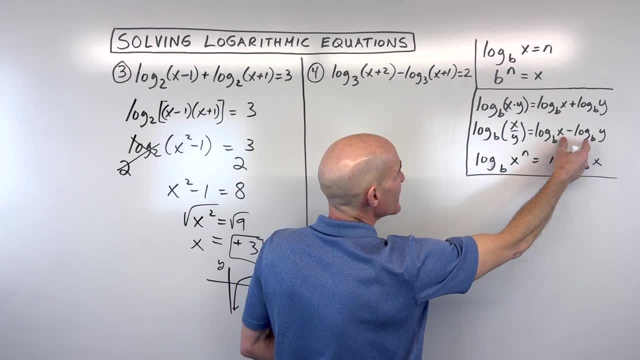 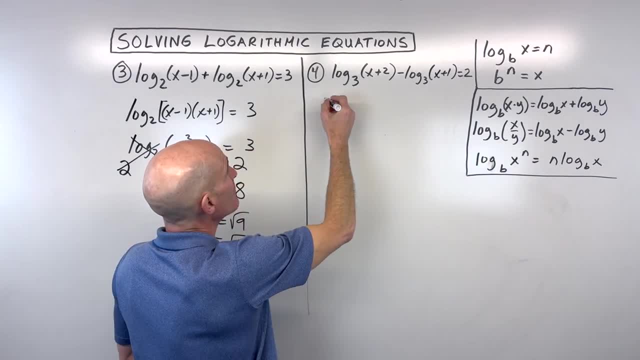 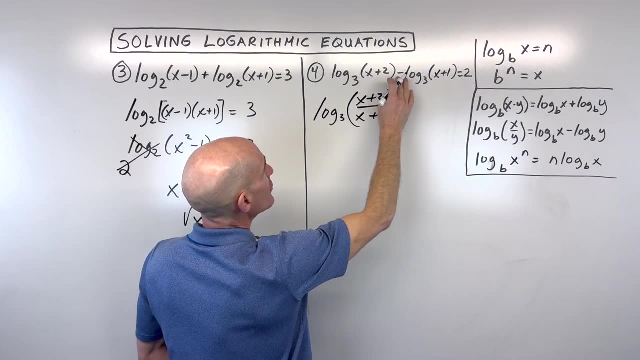 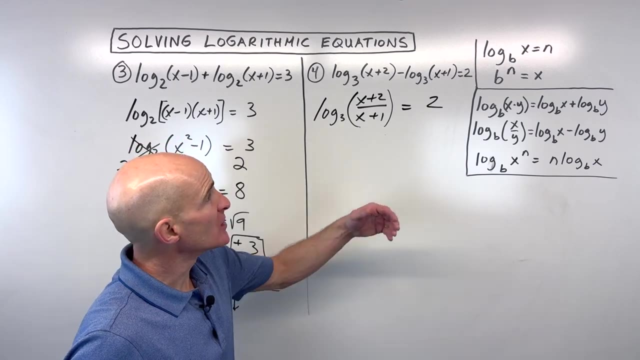 subtract, we divide the arguments right. So we're going to combine this into log base 3 of x plus 2, divided by x plus 1.. Remember the log that you're subtracting that argument goes in the denominator and this is all equal to 2.. Now what we can do is we can use our technique of switching it from the 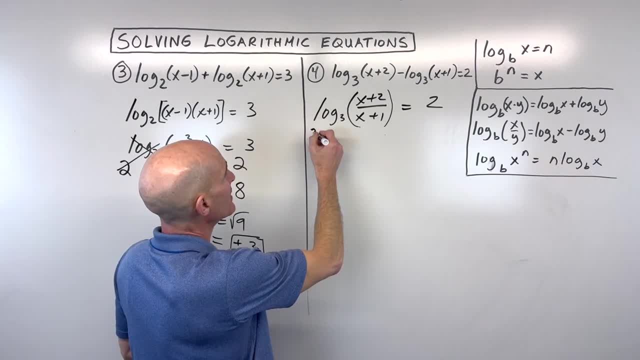 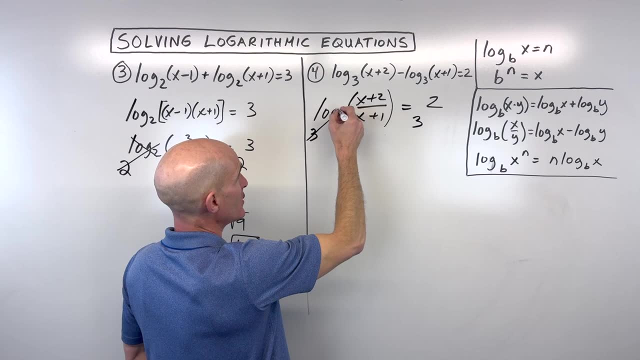 logarithmic form to the exponential form. Again, the way I like to do that is I like to exponentiate or raise both sides using that same base. So we've got an exponential function with base 3, a logarithmic function with base 3.. Those are inverses. They cancel one another out and we're 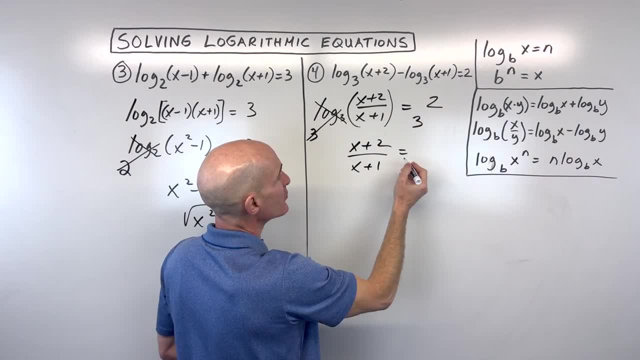 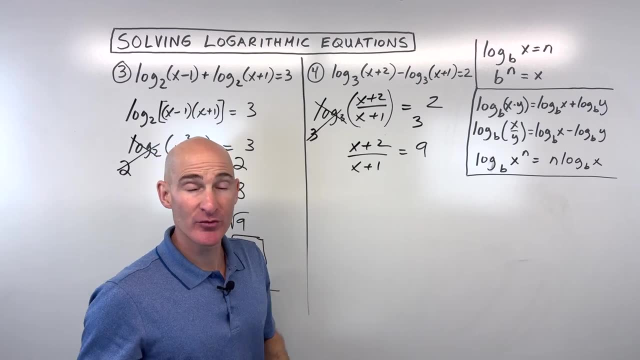 just left with x plus 2 over. x plus 1 is equal to 3. squared 3 times 3 is 9.. Okay, now we've gotten rid of that logarithm. We've got the variable a little bit closer to you know, being by itself here. 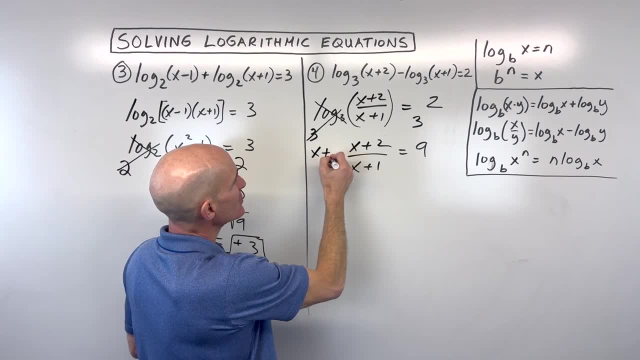 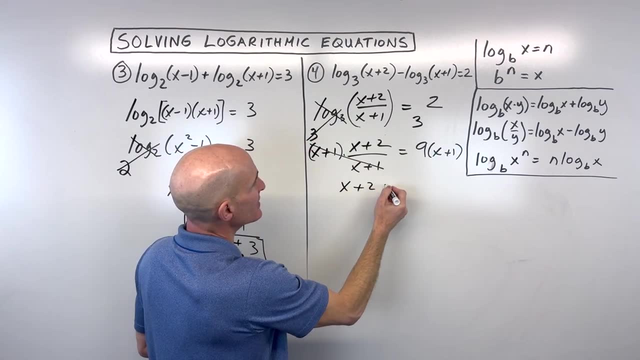 So now, at this point, you probably know what to do to solve this equation. I'm just going to multiply both sides by x plus 1.. I'm going to do a little bit of a spreadsheet to get rid of the fraction here, And we're left with let's. 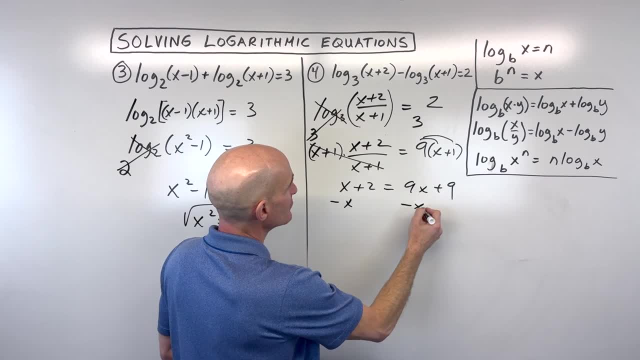 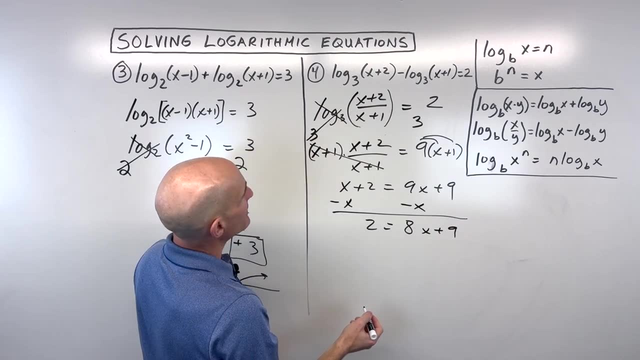 see: x plus 2 is equal to 9, x plus 9, and let's see we're getting closer. Let's subtract x from both sides. That comes out to 2 is equal to 8x plus 9, and let's subtract 9 from both sides. 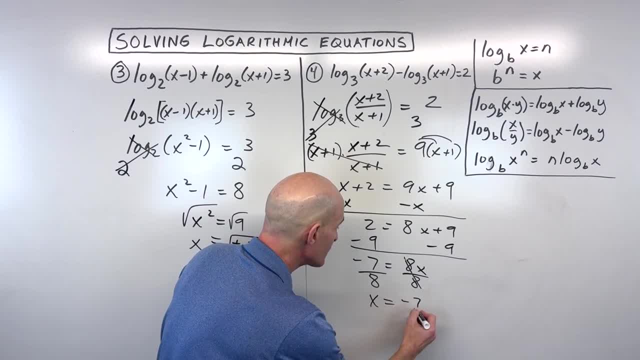 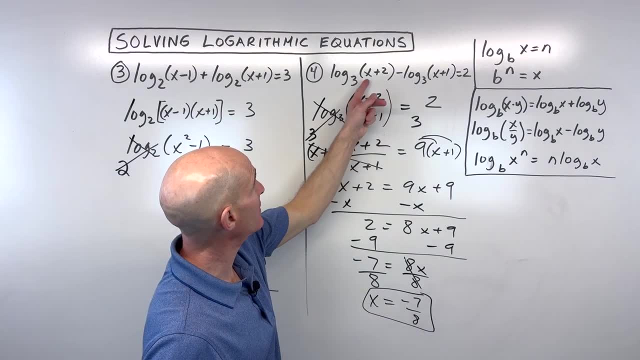 So now we get negative, 7 is equal to 8x. Okay, so x comes out to negative 7, 8.. And again we want to check that to make sure we get rid of the fraction. And again we're left with sure that it's a good solution, it's not extraneous. So if we go back here, negative seven, eighths. 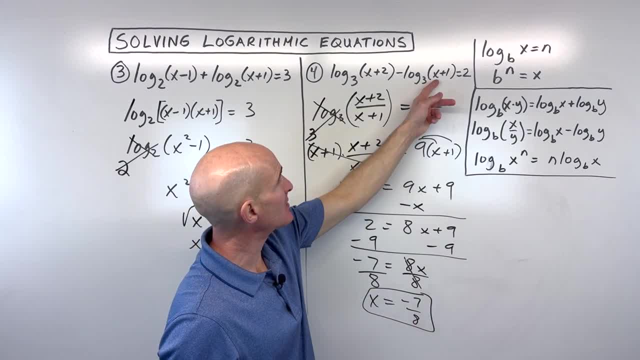 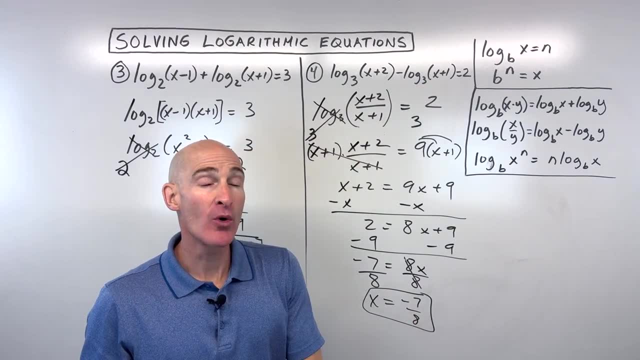 plus two, that's positive, that's a good value. Negative seven eighths plus one, that comes out to positive one eighth, that's a positive value. So negative seven eighths is a good answer here. Let's go on to one more example. Okay, for number five, we've got log base. 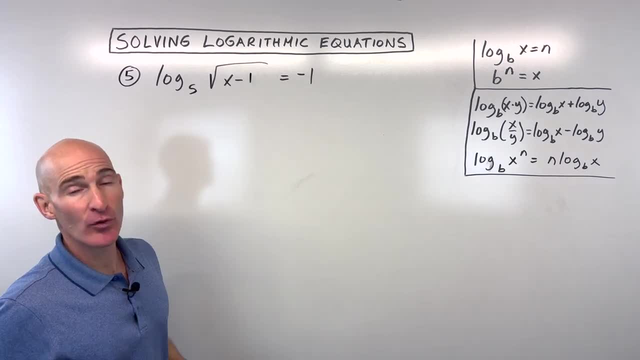 five of the square root of x minus one is equal to negative one. How would you solve that one? Well, I would do that same technique of raising both sides using base five or exponentiating. these are inverses and we're left with square root of x minus one is equal to five to the. 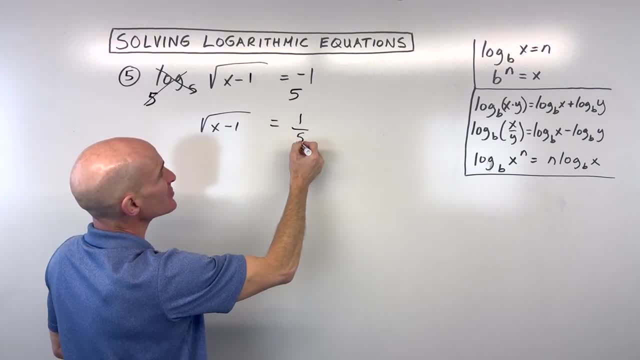 negative one. Remember that negative exponent tells us to take the reciprocal, so that's going to come out to one fifth. Now here we can square both sides, And one fifth squared is 125th. Here the square and the square root undo one another, So we're left with x minus.